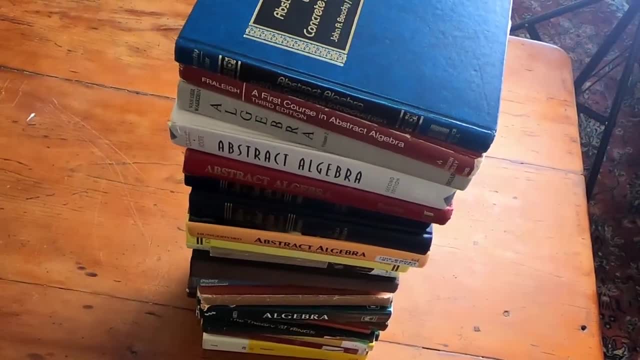 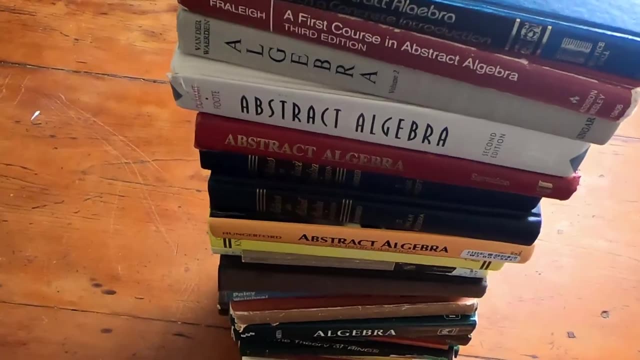 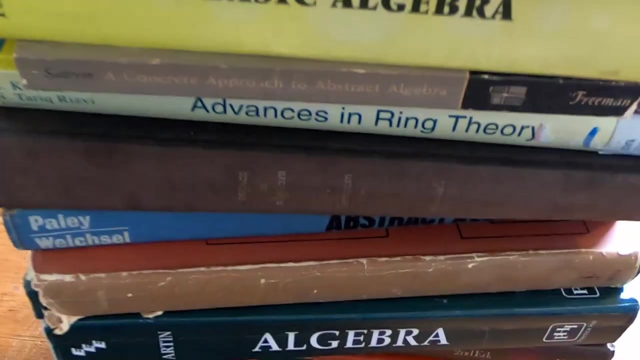 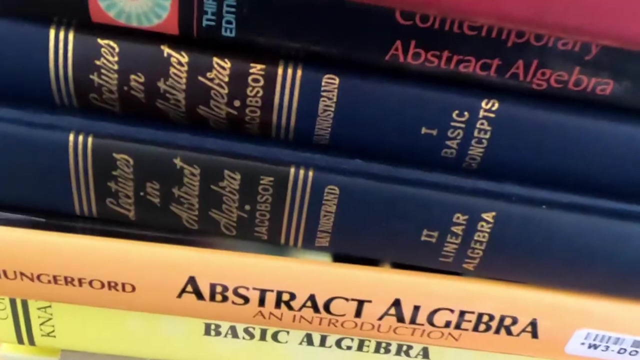 In this video, I want to go over some of my abstract algebra books. I think this is most of them. I'm pretty sure that I have more, but this pile here that you see is a collection of some, or maybe all, of my abstract algebra books. Now, again, I'm pretty sure I have more. These are just some of them. So in this video, we're going to go through and we're going to look at each and every single one of these books briefly. 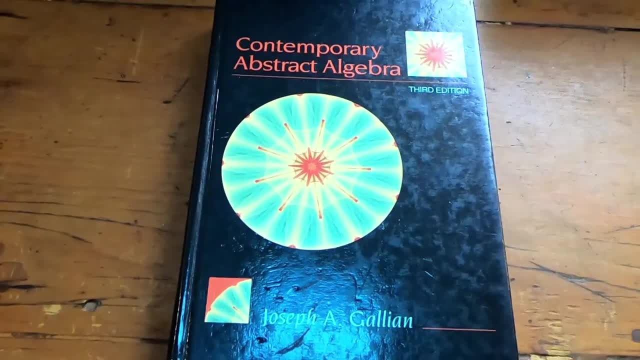 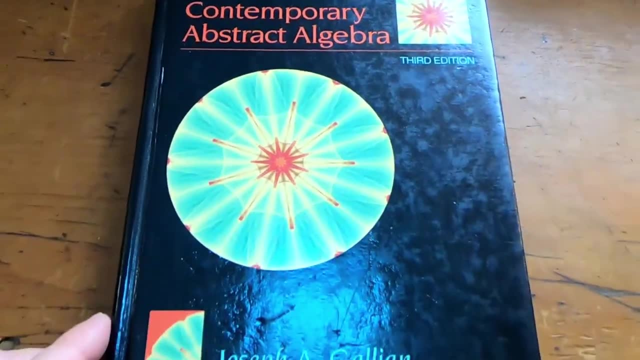 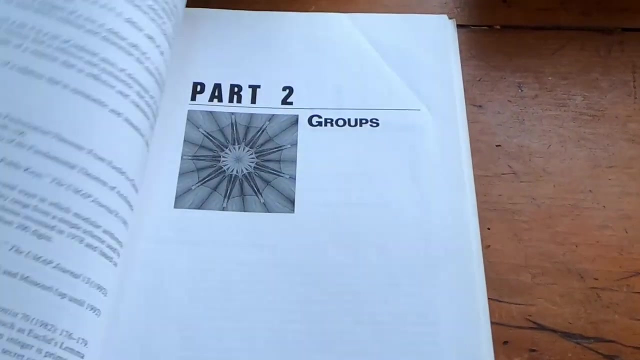 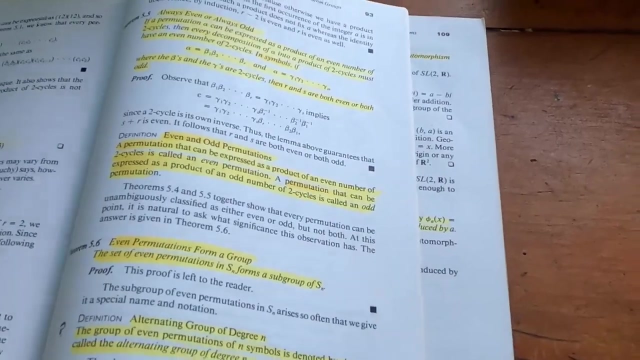 Okay, let's start with this book here. This is the Galleon book. If you're familiar with my book reviews, you may have noticed I've done a book review on this book already. The Galleon book is a really good book, and this is a special book to me because my good friend from New Zealand recommended this book. This book has a lot of examples, and I always think of the Galleon book as a book of examples. This is a good choice for beginners. It's contemporary abstract algebra. 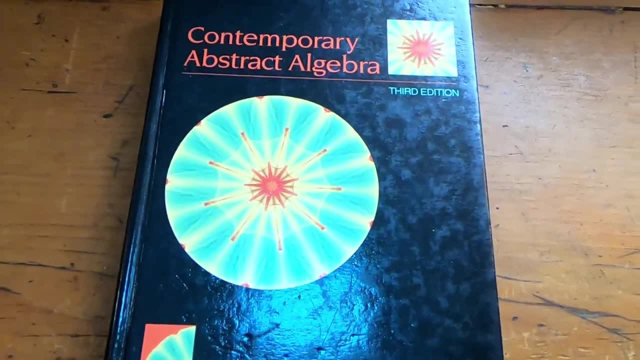 Okay, so let's get started. By Joseph Galleon. Let's keep going because we have quite a few books in this video. 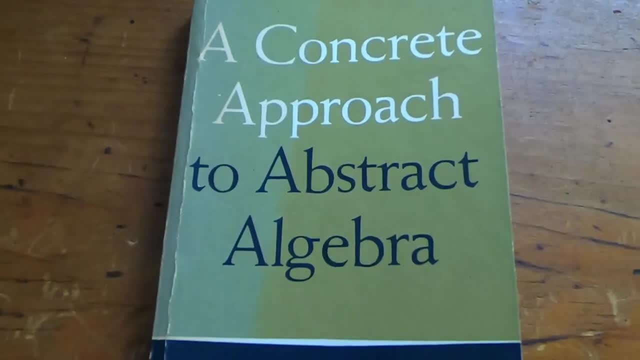 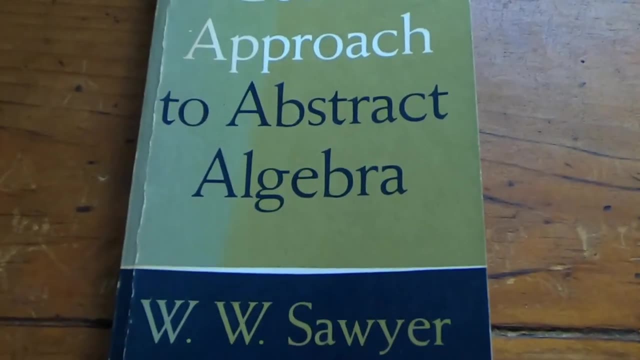 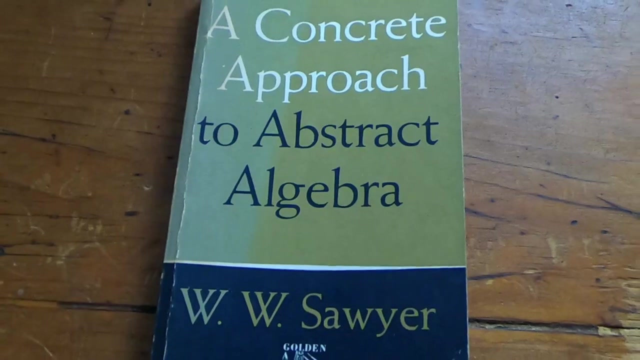 This next book was a gift from a former colleague. It's A Concrete Approach to Abstract Algebra by W. W. Sawyer. This is also a beginner book. I wouldn't say it's a fantastic book, but if you are looking for an additional resource and you have a few dollars to spare, check it out. It's a pretty decent read. I've maybe spent maybe 30, 45 minutes reading this book 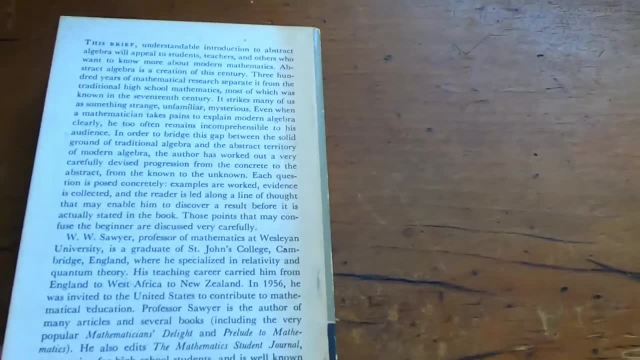 and perusing through this book. I never use it for a course. Again, this one was purely a gift. 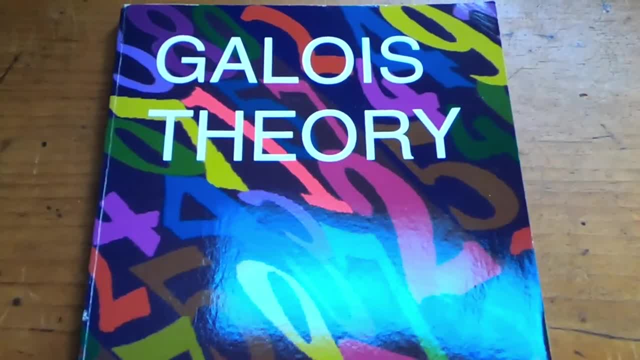 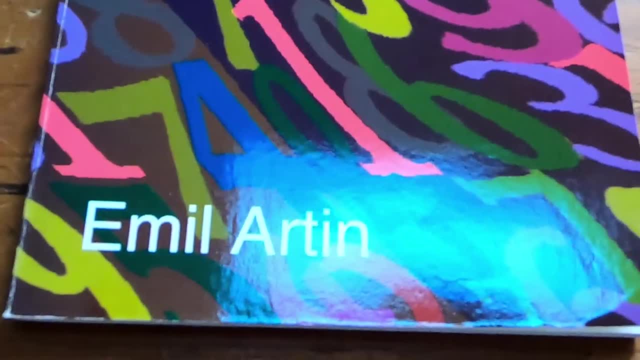 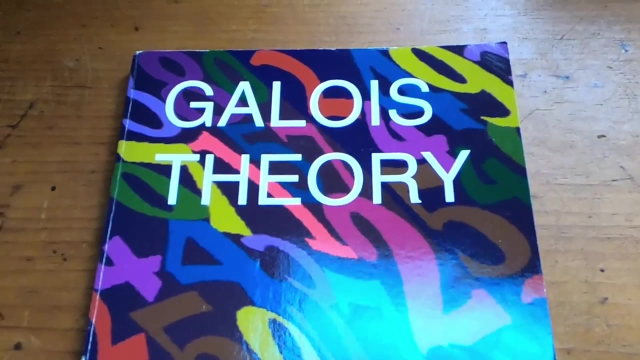 This book was written by a very famous author. This is Galois Theory, written by the one and only Emil Aarten. These are a transcription, I think that's the right word, of his notes when he used to teach at the University of Notre Dame. I believe this is one of the first ever written books on Galois Theory. 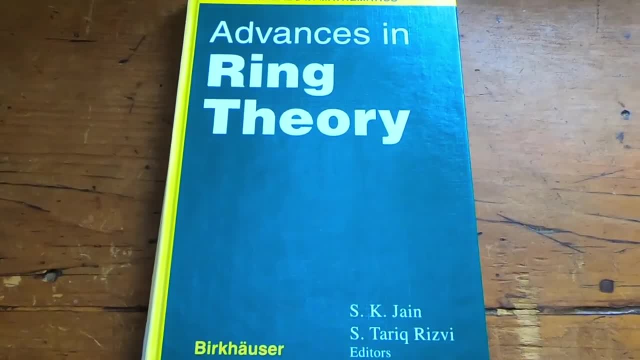 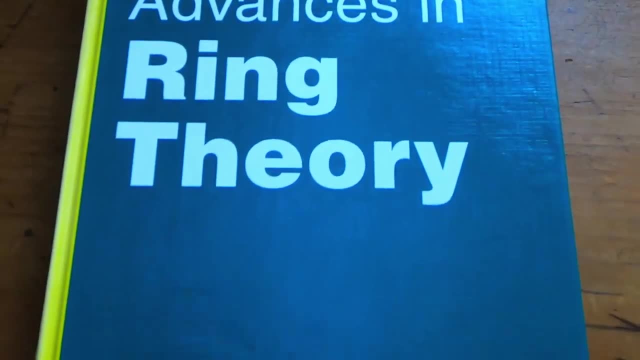 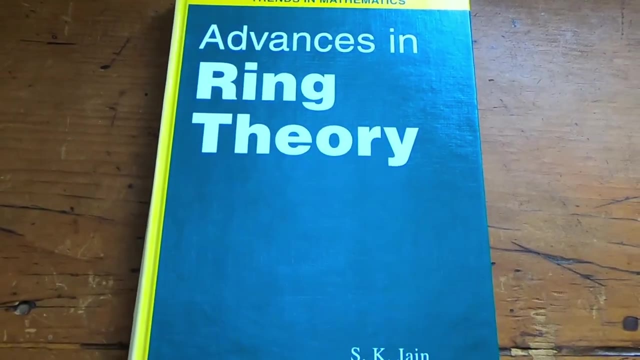 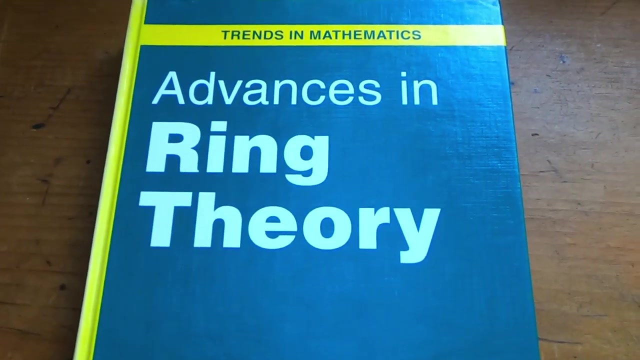 This next book is extremely high level. In fact, this is it. This is as high level as you can get. So, Trends in Mathematics, Advances in Ring Theory. This is research level mathematics here in Ring Theory. This is a collection of papers that were presented in 1996, May 1996. And so, it's just research level math in Ring Theory. It is extremely hard to read. It is not for beginners. But, if you're interested in getting a glimpse at what's in there, you can go to the link in the description box below. So, this next book is extremely high level. In fact, this is it. This is as high level 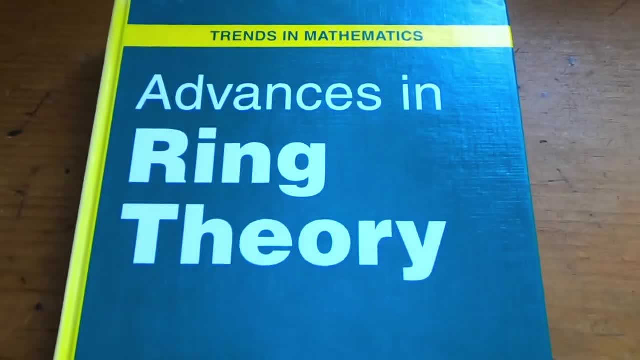 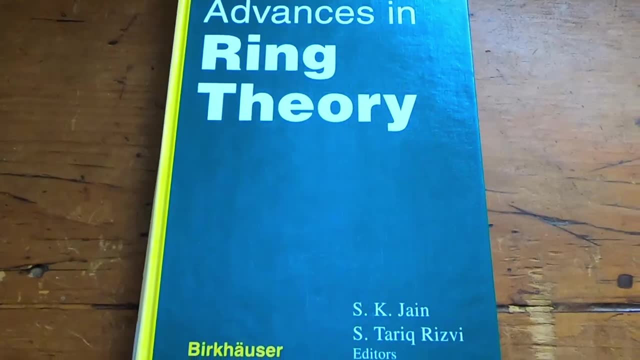 as you can get. Some of the research actually is. You can attempt to read this book. When you read this book, you'll have to probably reference many other books to understand what's going on because, again, this is research level abstract algebra. 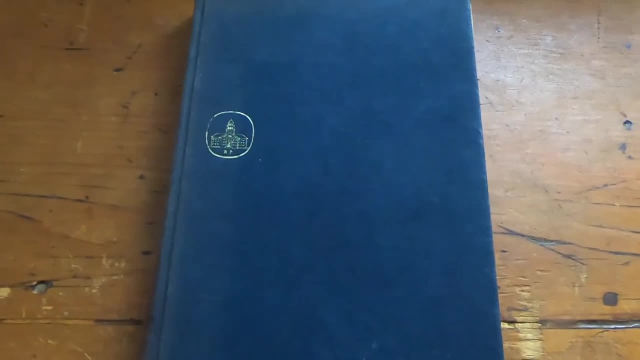 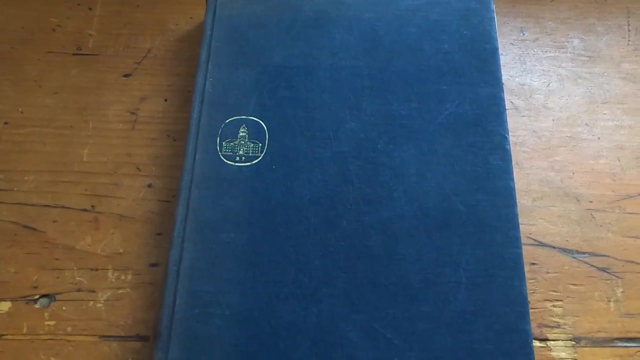 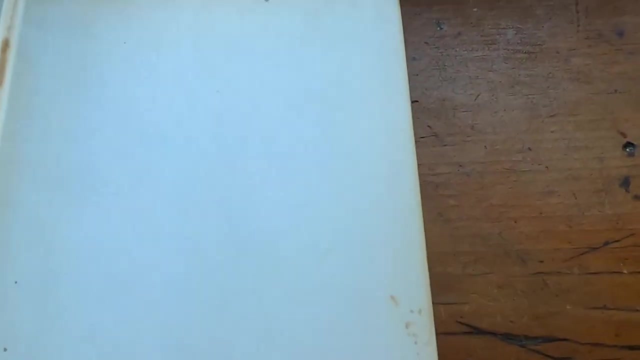 This next book is the book by Israel Nathan Herstein, Topics in Algebra. This book is ultra famous. Had a good friend in graduate school who absolutely worshipped this book. And with good reason. This is a fan book. This is a fantastic book for beginners and for experts alike in abstract algebra. 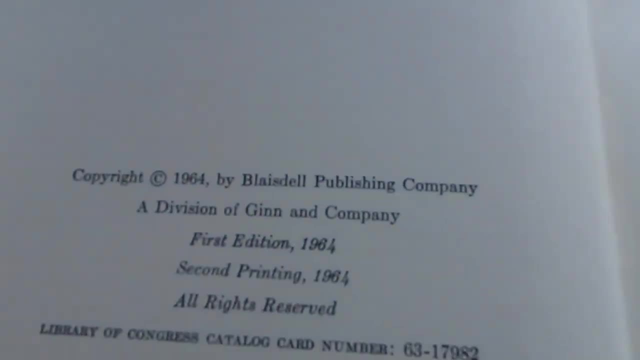 I would consider this an advanced beginner book. Again, the book is Topics in Algebra, written by the great Israel Nathan Herstein. 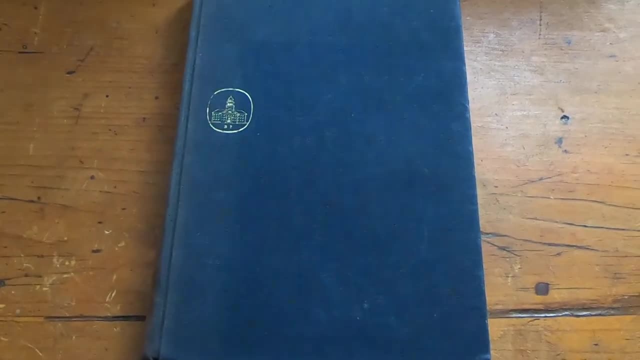 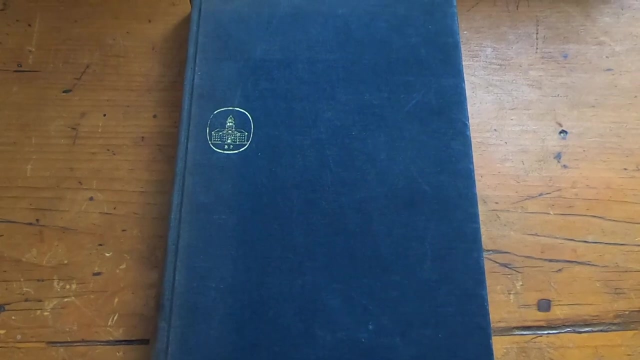 And I've mentioned this before, but if you haven't seen the video, I'll mention it again. Coincidentally, the author of this book went to the same grad school I went to. So that always leaves a special place for me. This book is great. 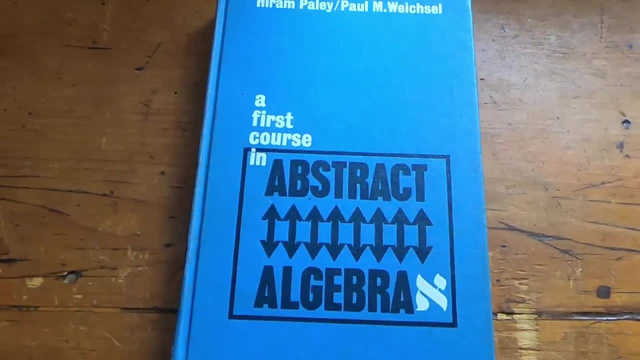 This next book is extremely good. And I have actually read most of this book and I have referenced it. 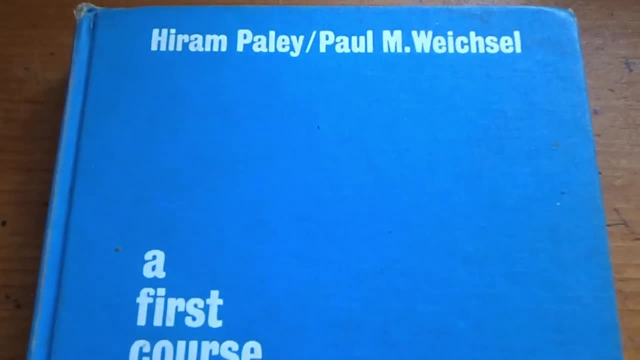 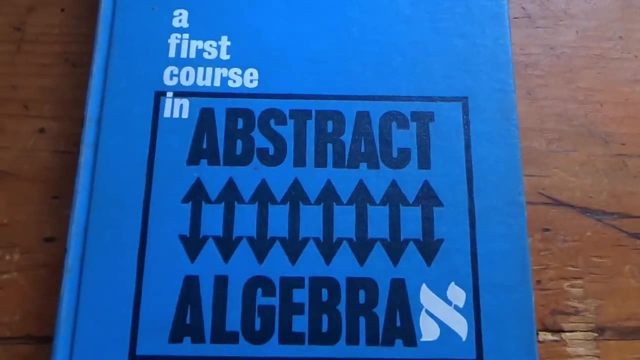 I have not done a review on this book on YouTube yet. The book is written by Hiram Peli and Paul Weichel. It's a first course in abstract algebra. 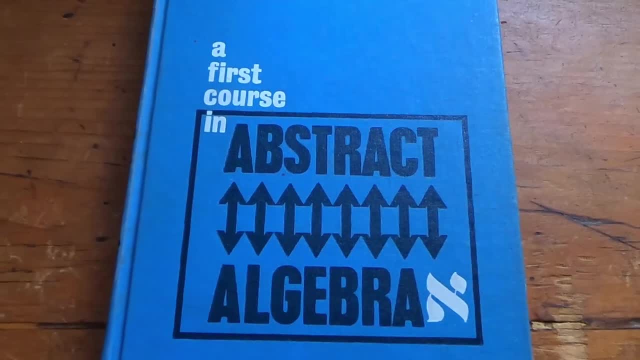 It is a beginner book, but it is written at an advanced level and it does have some higher level examples. It's extremely good. I have a lot to say about this book. 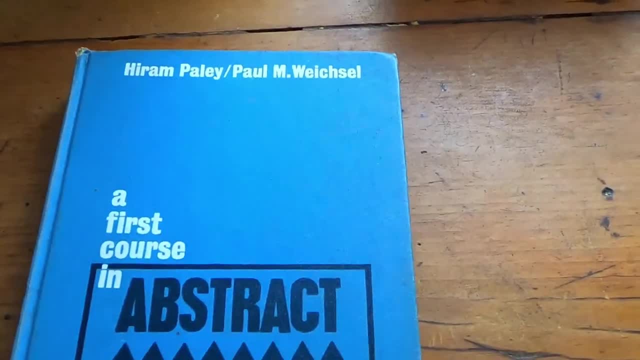 I really like this book and I will be doing a review on this book in the future. 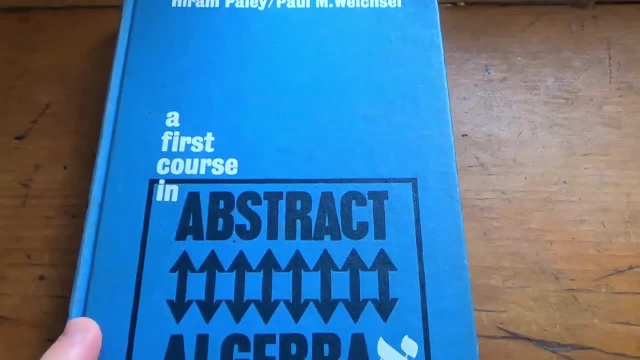 One negative about this book is the function notation. But I'll save that for the review and I could spend 10 minutes talking about this book. 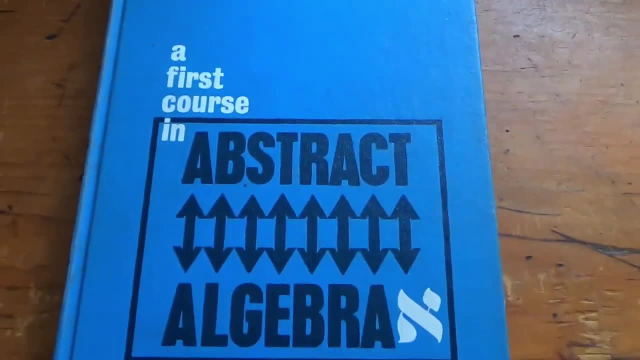 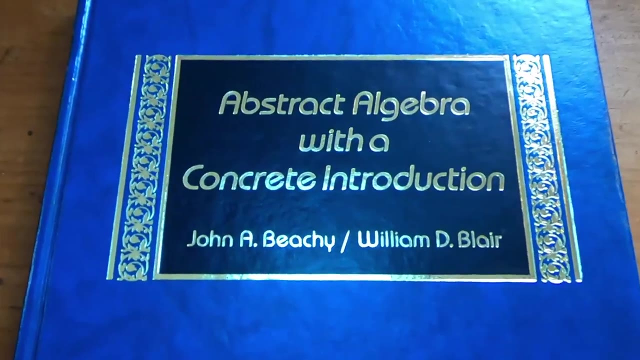 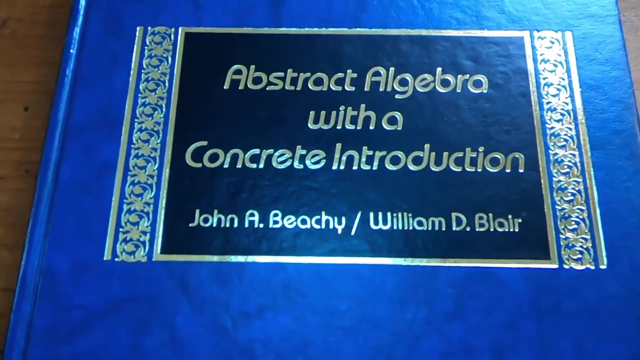 So again, it's Peli and Weichel, a first course in abstract algebra. This is one of my favorite books in abstract algebra because this is the book that I used to teach myself field theory. So I learned field theory online. And I learned it on my own with this book. It took a lot of effort. I had to start with the chapter on polynomials. 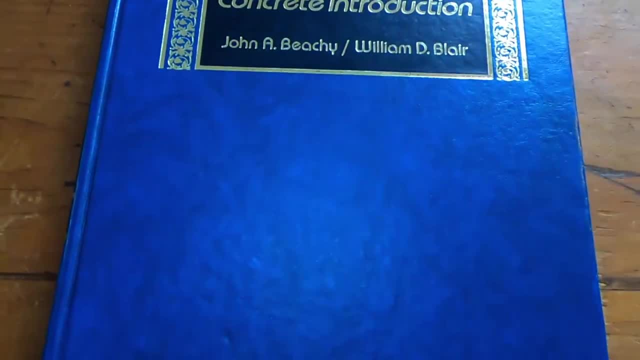 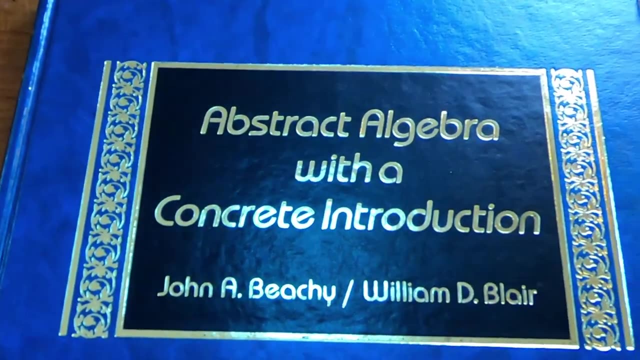 This is a beginner book in abstract algebra and it's a good book, but again, I've mainly used it for field theory and also I referenced it for CELO theorems group actions as well. 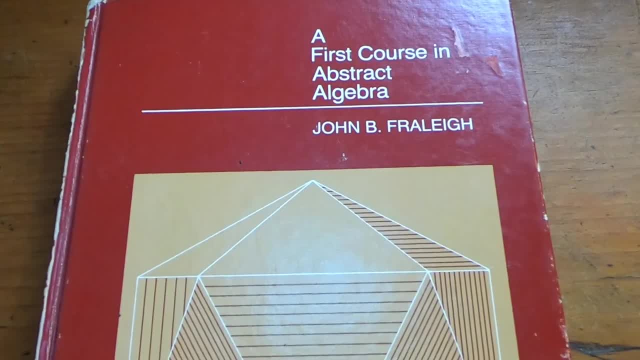 The Frillet book is a book that I bought because my first course in abstract algebra teacher said that I should buy it. So I did. 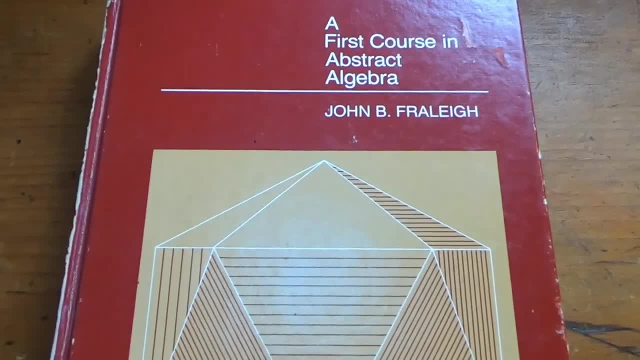 And I was very happy with it. This is a beginner book. 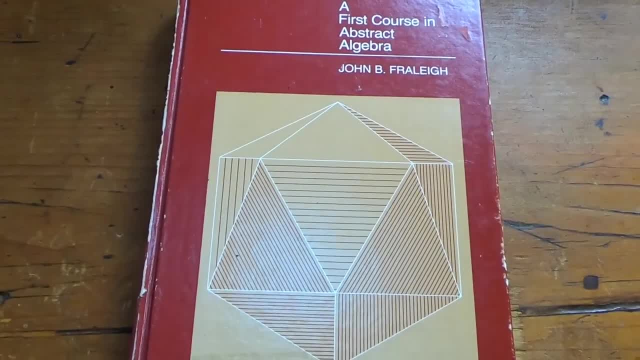 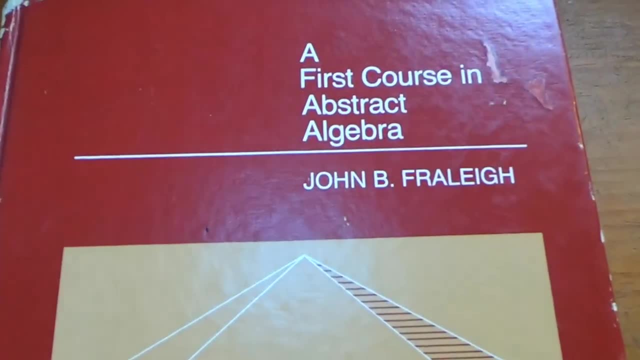 It moves at a really quick pace. But it's written at a really nice level. This book is a pleasure to read and is probably one of the best abstract algebra books ever written. 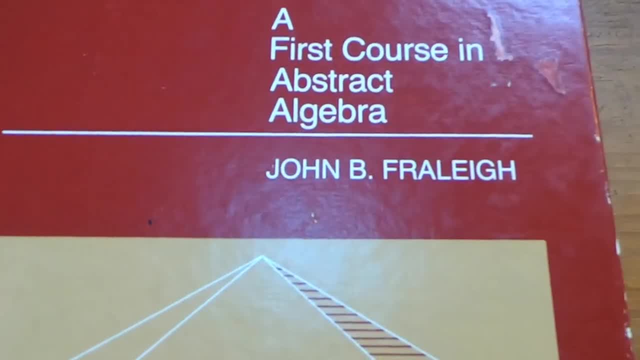 I highly recommend it if you're looking for a beginner book in abstract algebra. 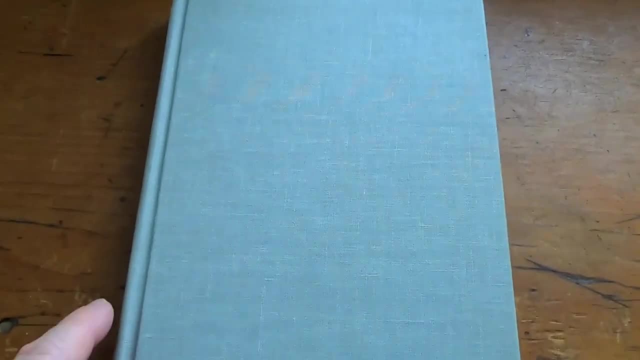 This is an abstract algebra book that kind of has a legacy associated with it. I have not done a review of this book. 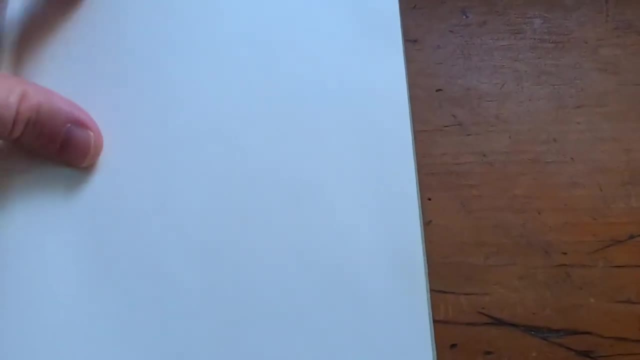 Let's look inside it. This book is really old school. I bought this because... I read on the internet on some forum years ago that this was considered a classic in the subject. I thought, oh, I should buy this book. So it's algebra. This is volume 2. I do not own volume 1. Not yet. 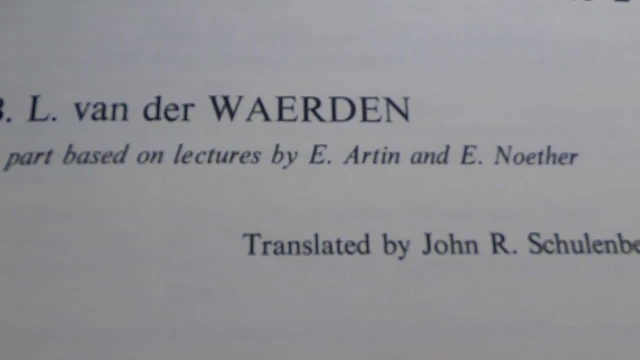 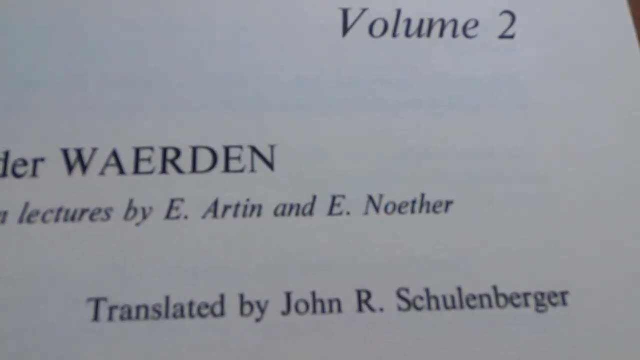 And it's the van der Waarden book. And in part based on lectures by E. Arten. Yep. That's the guy who wrote the Galois theory book that we just saw. And E. Noether. That's Emmy Noether. That's the same Noether after which Neutherian rings are named. 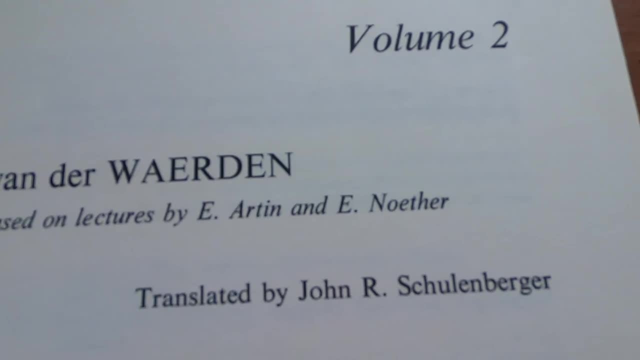 So this book is very close to the source. Arten was probably one of the first people ever to write about Galois theory. Emmy Noether created some amazing mathematics. She was an amazing mathematician. 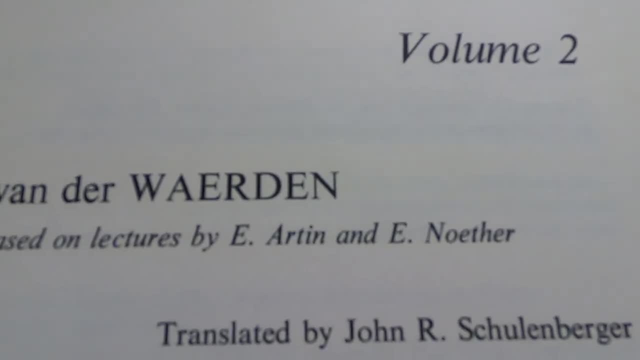 So van der Waarden was very close to these people. So it's kind of interesting. It's kind of like you're reading some of the masters when you're reading this book. 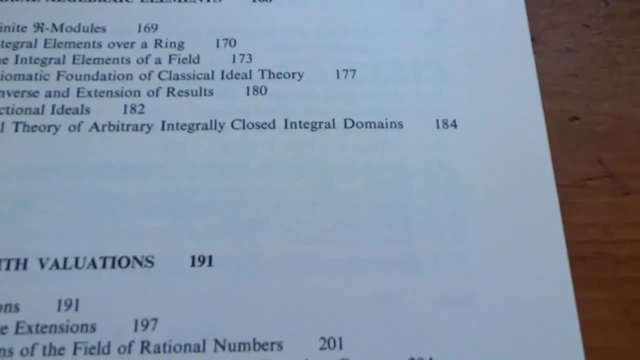 The negative thing about this book is a lot of the notation is pretty hard. He uses those fancy German letters. There's a lot of notation that you won't see in a lot of books. 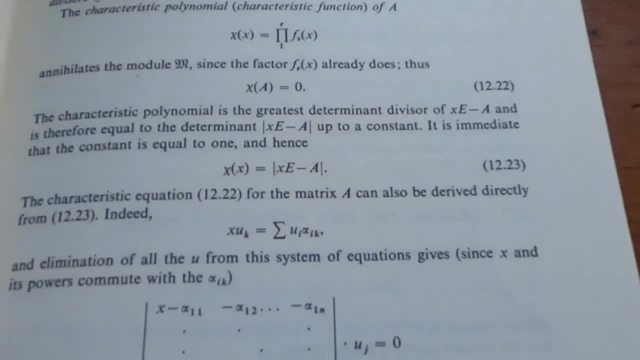 So it does take some getting used to. 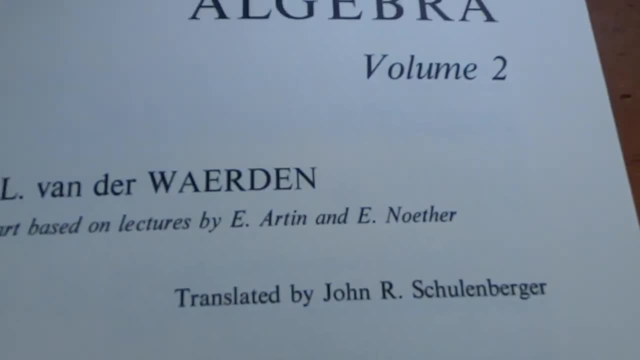 But nevertheless, again, the book is van der Waarden. And it's considered a classic in the study of abstract algebra. 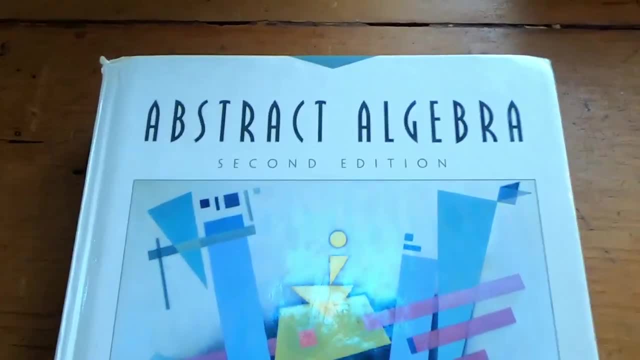 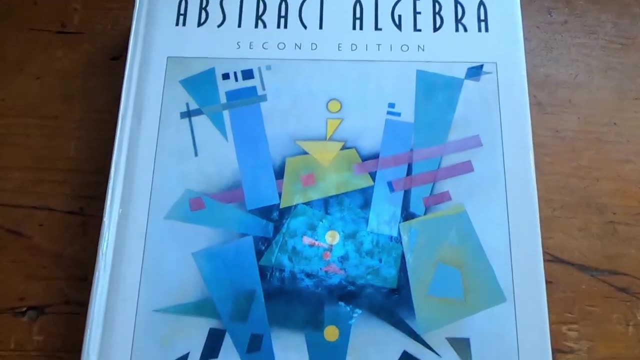 This next book is absolutely amazing. This is the Domet and Foot book on abstract algebra. This is probably the best graduate reference. I mean it's such a good reference. This book has pretty much everything. 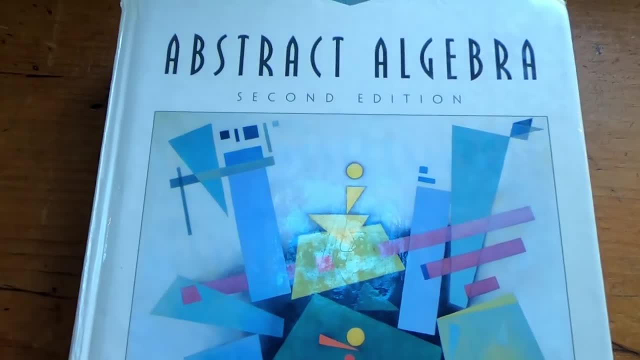 It covers all the topics in a very standard way. So if you're taking an abstract algebra class, either as a graduate student or an undergraduate student, 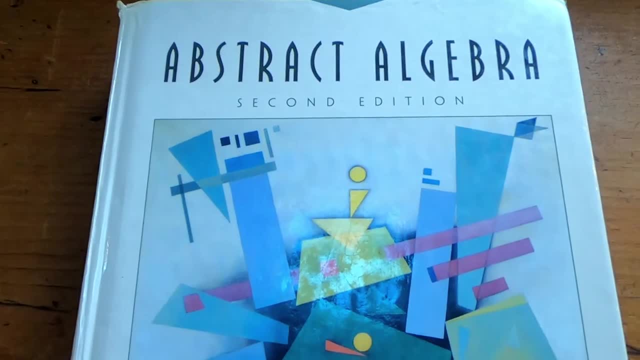 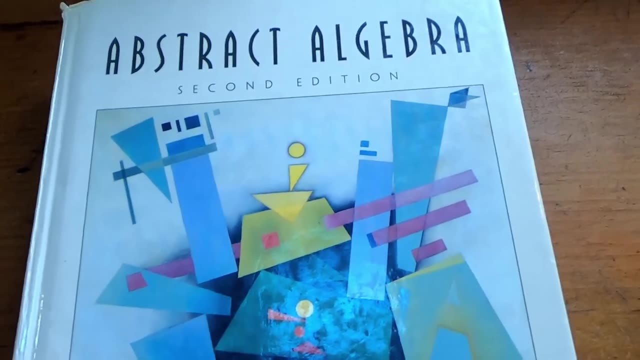 the Domet and Foot book will serve you well because it's an excellent reference. I love this book. And my main regret with this book is not getting a newer copy. The binding is messed up in this copy. 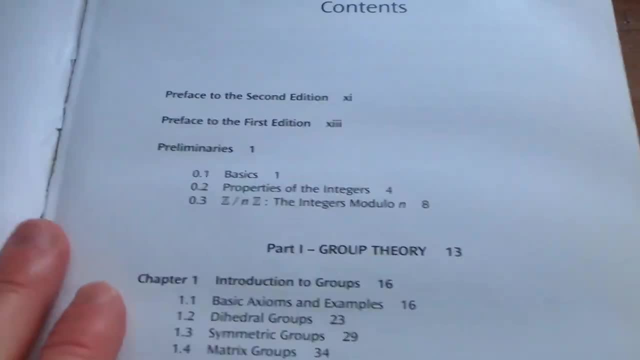 Let me show you. Let me open it so you can see what I mean. 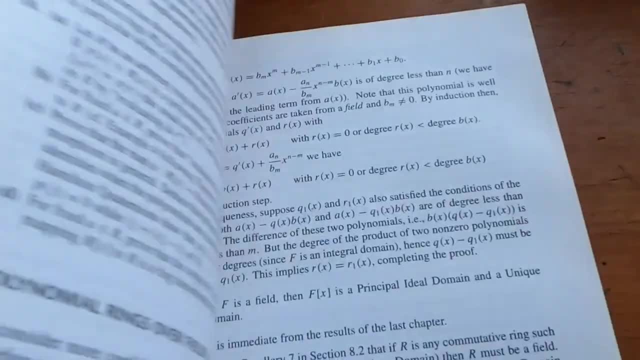 See there? It's cracked. And some of the pages, let's see. Yeah, the pages aren't falling out. 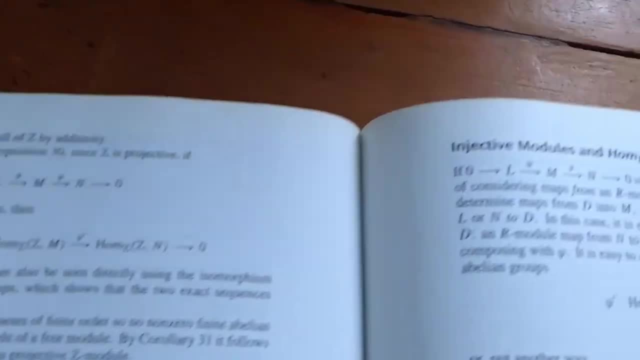 I do have issues with it. It's not in the best condition. It's a great book. 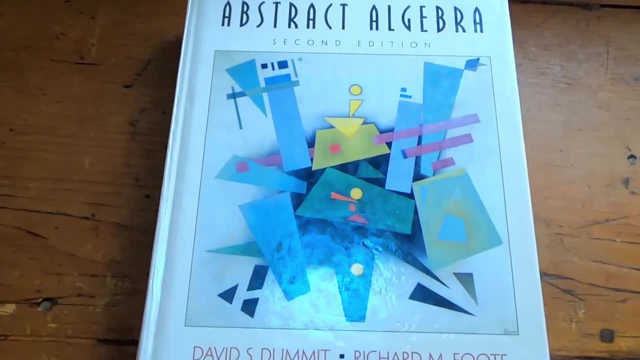 And if you're learning abstract algebra or if you're looking for a reference book, I highly recommend this one. This is the book that I used when I first studied abstract algebra. 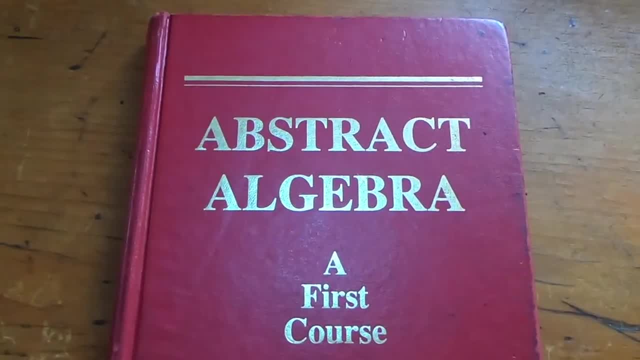 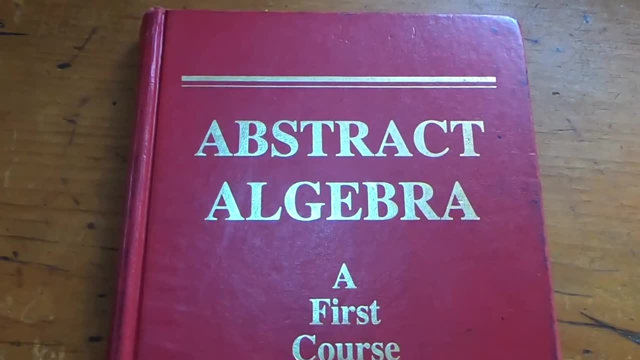 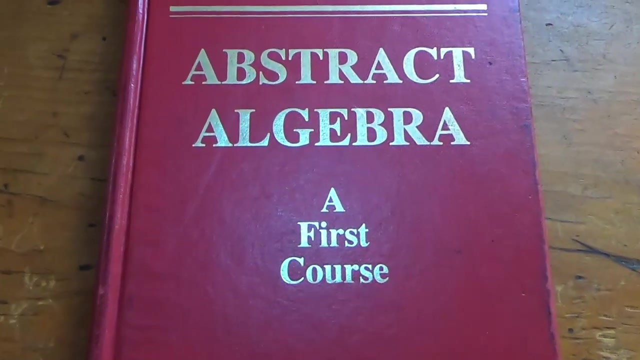 It's a pretty good book. It's a very gentle read compared to the other algebra books I have. It's probably the easiest one to read. It's the Saraceno book. I've actually read this entire book. Every single page. I've done, I would say, maybe 80% of the problems. Maybe even 90%. I've done most of them. 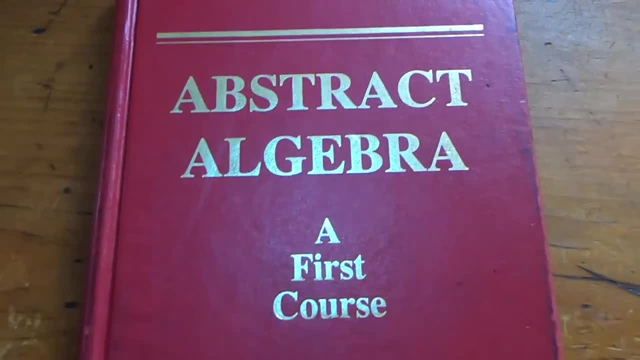 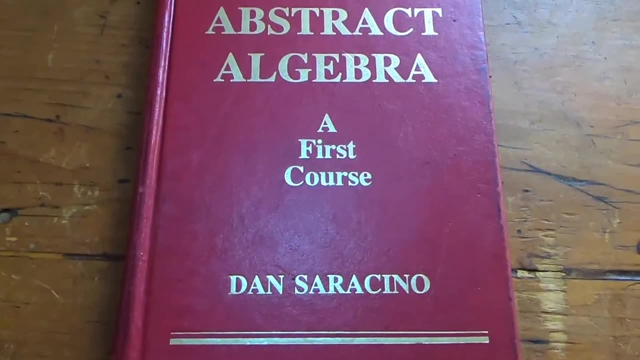 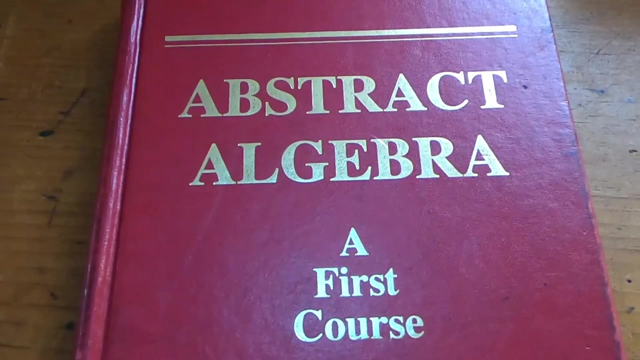 The only negative I have to say about this book is that it's not comprehensive enough. You know, you get to the end of the book and there's still a lot more to learn. Nevertheless, it's a really, really good book. And Saraceno does a great job explaining. If you're looking to learn abstract algebra, I think this is probably the best beginner book. Again, I might be biased. This is the book that I used. So, yeah, good book. 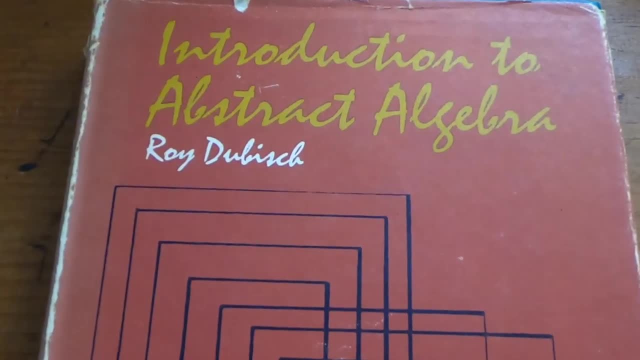 This next book is called Introduction to Abstract Algebra by Roy DeBish. 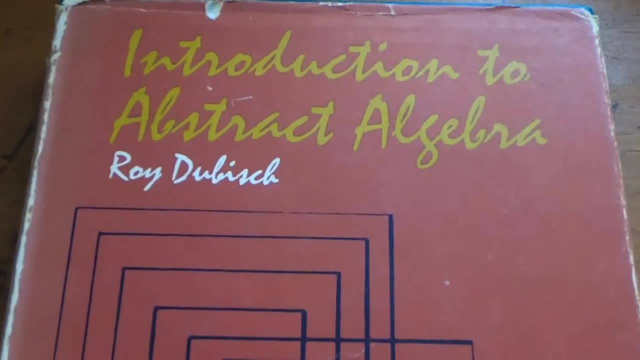 This book was a gift, again, from a former colleague. 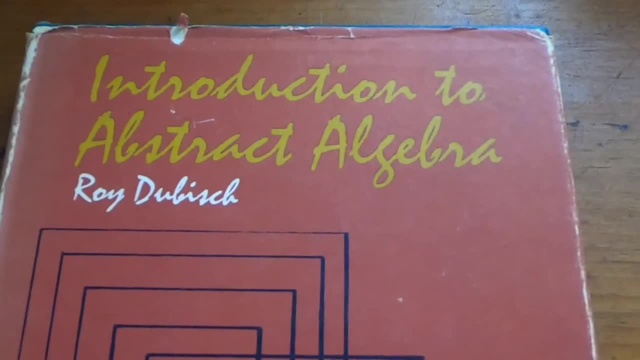 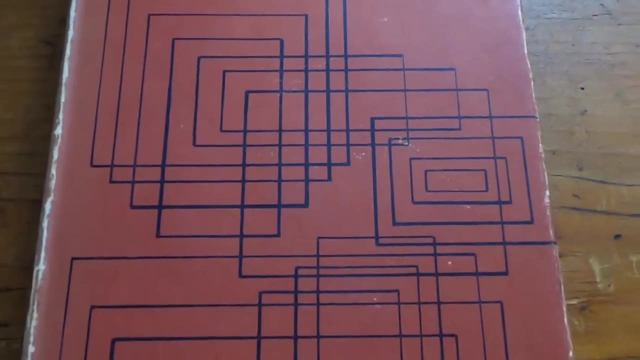 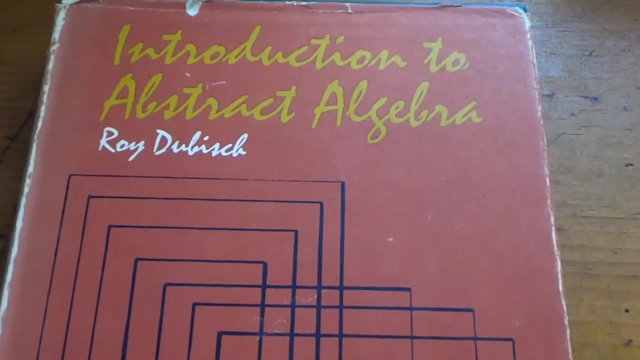 I'll be honest. I have only briefly glanced at this book. I've maybe read one or two of the sections. And I was quite pleased. It's a pretty good book. I wouldn't say it's as good as some of the other books like the Saraceno book or the Beachy and Blair book or the Galleon book or the Frele book. It's not quite to that level. But it's still a decent book. 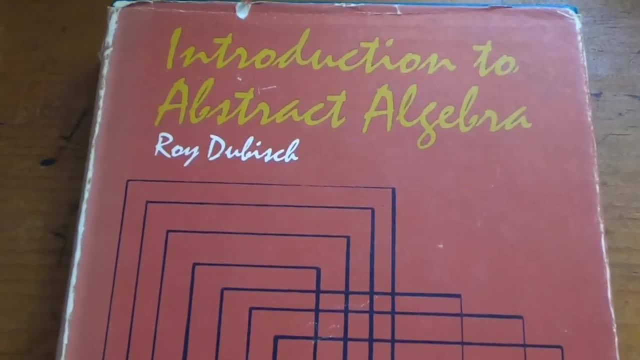 So if you're looking for another source, if you already have all those other books and you just want another book, this one is one to consider. I'll do a review on this book at some point in the future. Okay. 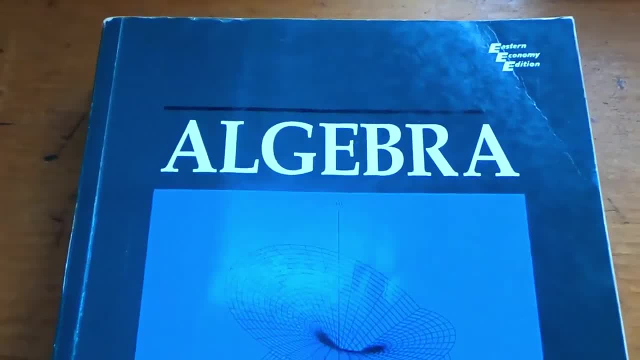 So this is a great book to read. But I didn't find it very good as a reference. 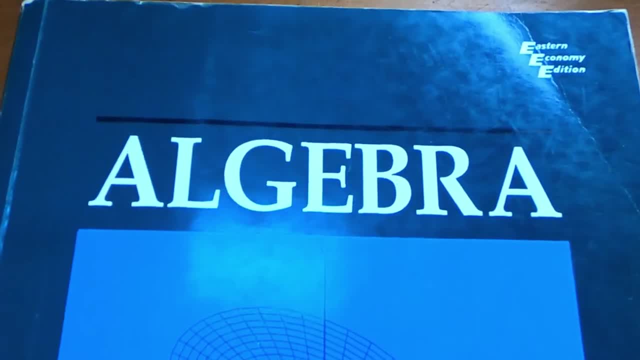 Perhaps the index is not done as good as it could have been. 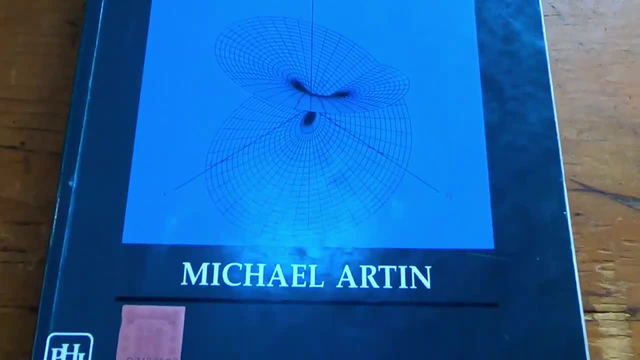 This is the book called Algebra by Michael Arten. And, again, it's an extremely good read. If you just want to browse. 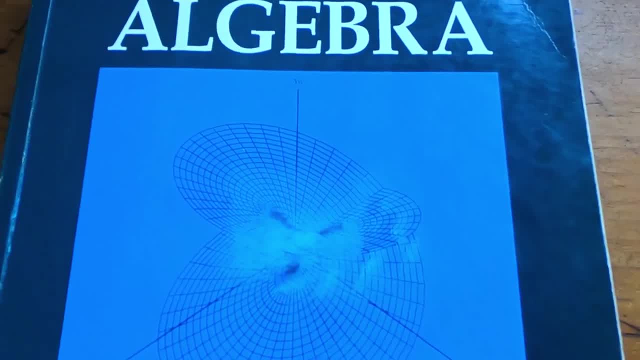 If you just want to buy a book to read and learn from, this is a good one. 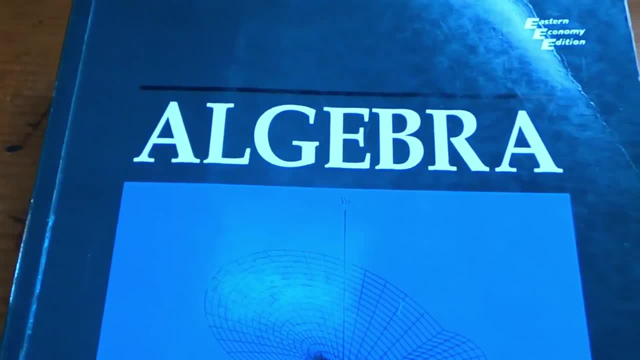 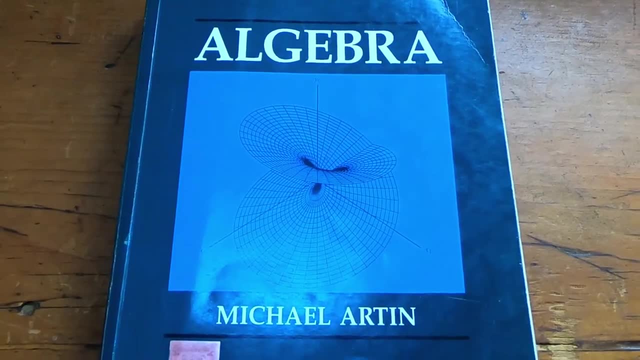 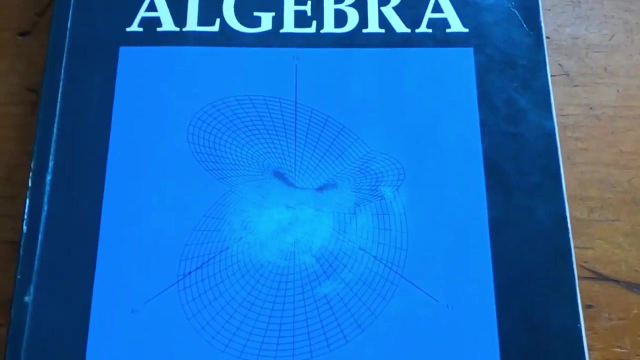 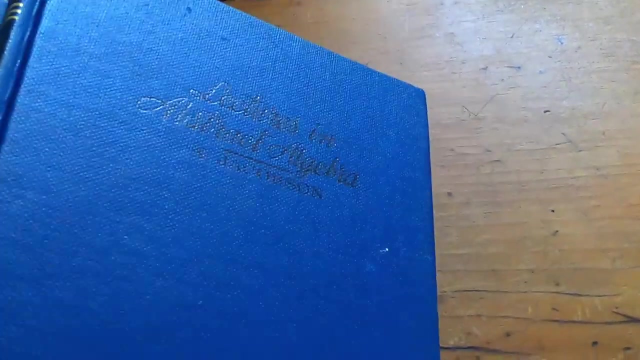 He takes a very linear algebra-centric approach to his mathematics. This is the son of Emil Arten. So Emil Arten is the guy who wrote the Galois Theory book. So Michael is his son. And I believe Michael works at MIT or he used to work at MIT. It's a great book. These are the lectures in abstract algebra by Jacobson. This is the same Jacobson. 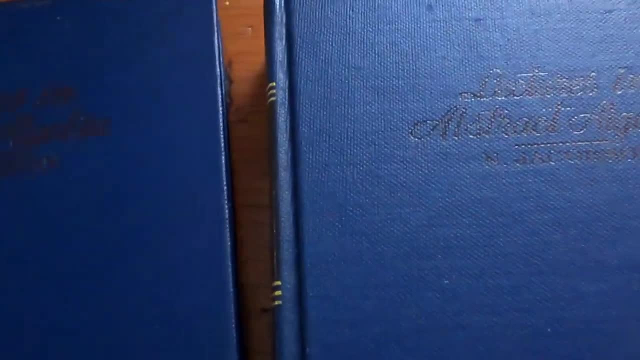 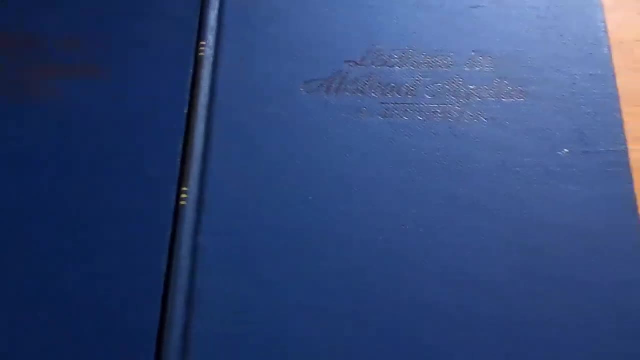 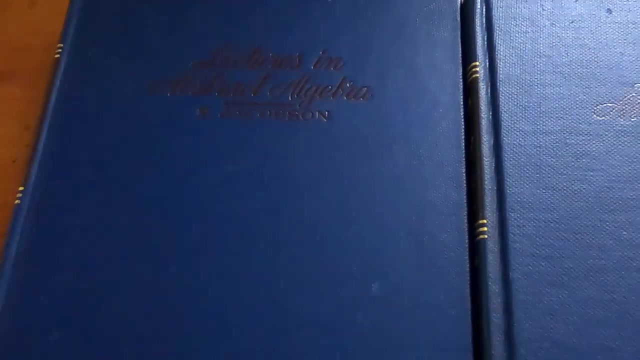 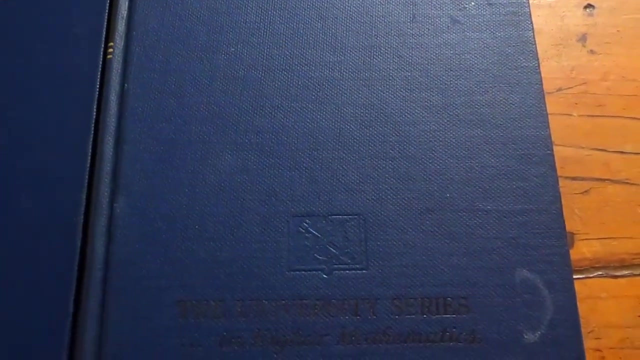 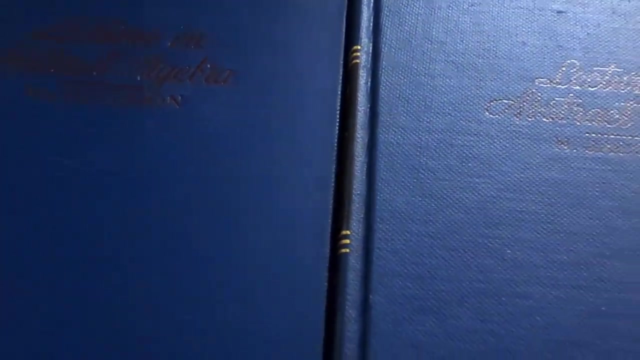 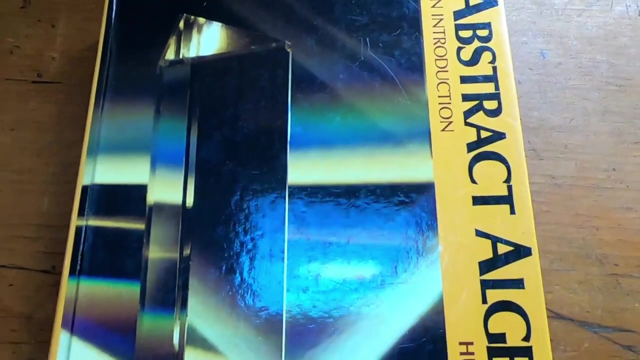 This is the same Jacobson for which the Jacobson Radical is named. I have used these books mainly for ring theory. So I referenced this when I was doing some independent study in Natharian rings and ring theory. So these books have some good information on that. So the notation in these books is a little bit hard to read. I don't know if newer editions still have that notation. But otherwise, I was really pleased with what I got from these books, which was the ring theory. This is the undergraduate version of Hungerford's book. This is a beginner book by all means. 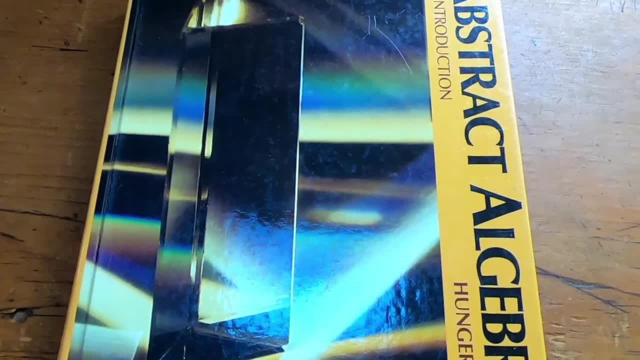 It reads at a very basic level compared to some of the more advanced books that we've discussed. It's a good book. 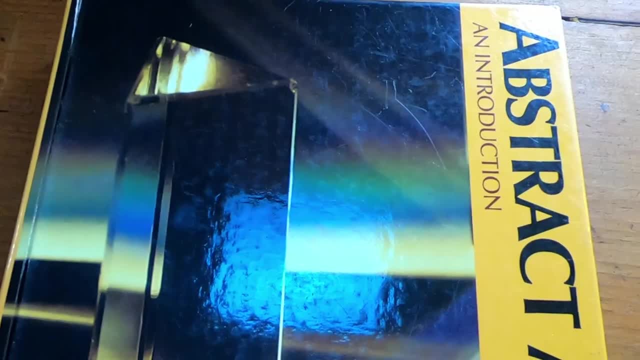 If you're looking for a supplement to an introductory book, then look no further. This one's really good. 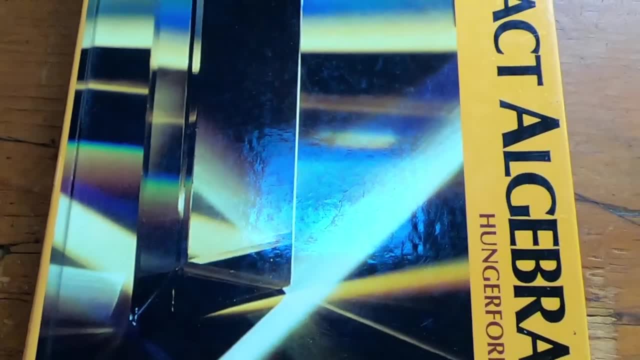 Hungerford also has a graduate-level book, which I honestly think is better. But again, this is... This is the undergraduate version. 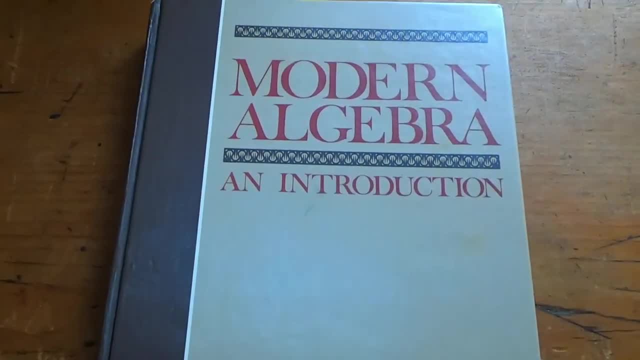 Yet another introductory algebra text. This one is called Modern Algebra and Introduction. 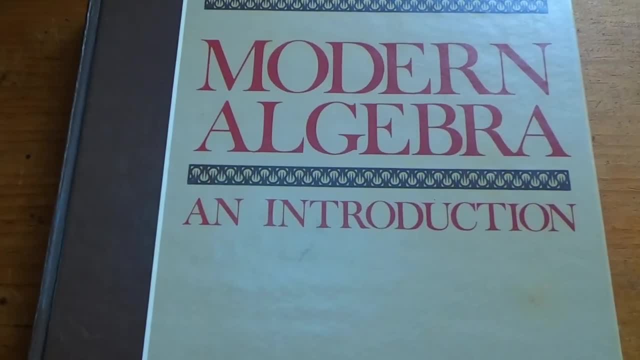 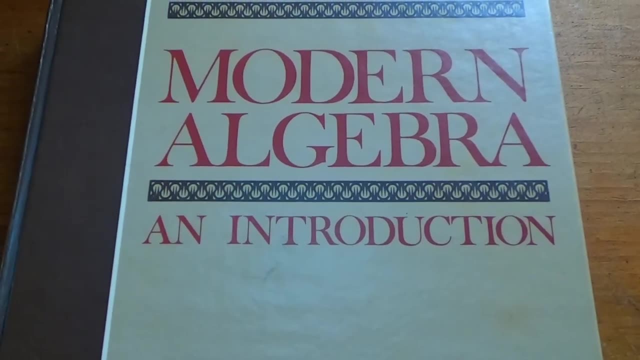 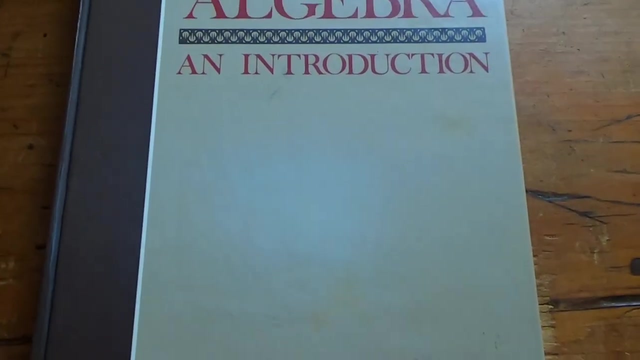 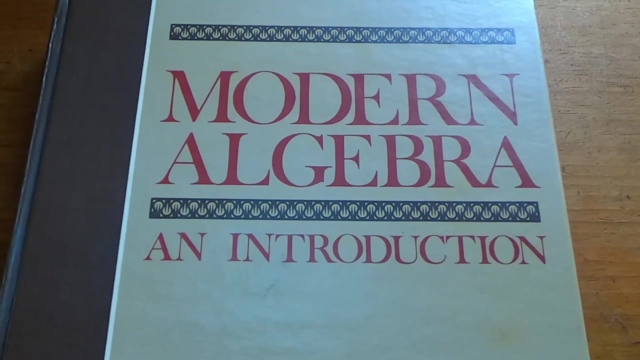 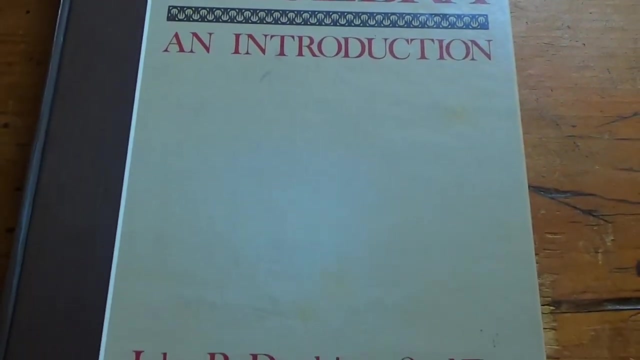 This one actually has some interesting applications of abstract algebra that you don't really see in any of the other books. Also, it just has certain theorems and things in it that you don't see in the other books. I have spent a decent amount of time working through this book. I think I've made a few videos from this book. Or at least I've planned a few videos. I've never made them. It's a really good book. I bought this when I first started learning abstract algebra as a supplement. And I did find myself reading portions of it and referencing it quite often. Again, it's the Durbin book. And it's Modern Algebra. 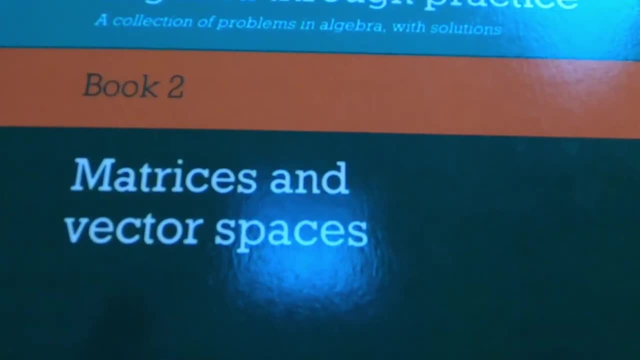 This next book is called Algebra Through Practice. And this is book two. It's on matrices and vector spaces. 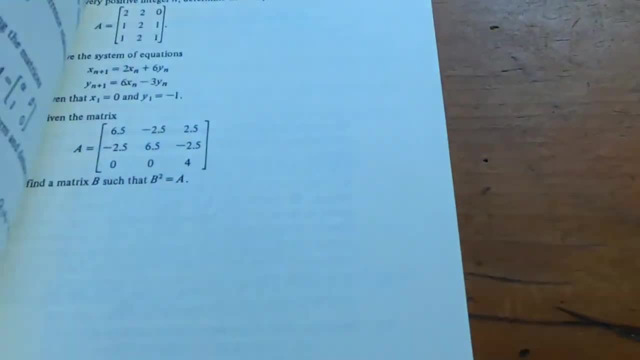 This is basically a book of full solutions. There are full solutions to every single problem in this book on matrices and vector spaces. 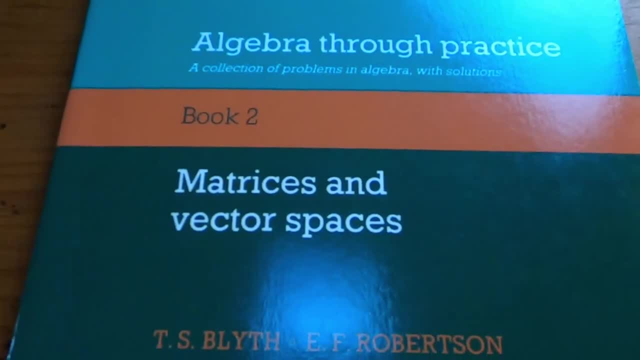 The number one downside of this book is that it is so expensive. It's not that inexpensive. 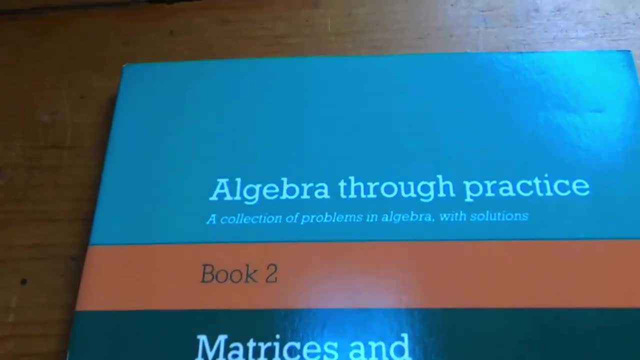 You can't get it for $5. I'm pretty sure I paid less than $10. But it has been several, several years. 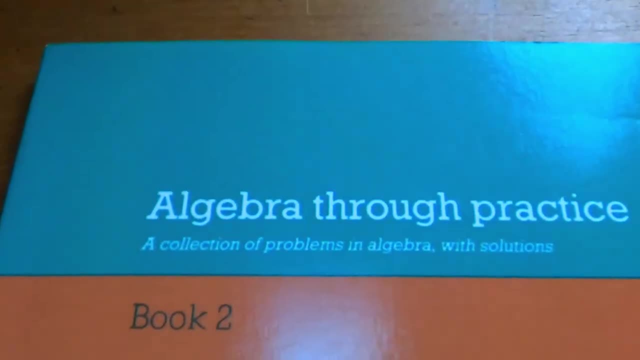 So it's the book on matrices and vector spaces, Algebra Through Practice. And it has full solutions. If you can get it for a few dollars, you know, totally, totally, you should just totally buy it. 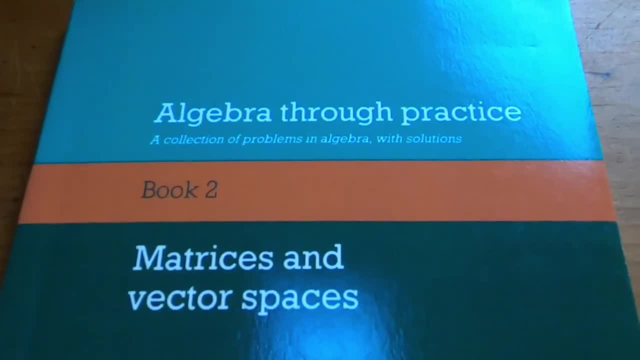 I have not been able to find it for only a few dollars since I bought this one. This next book is also Algebra Through Practice. And this is the one on groups. 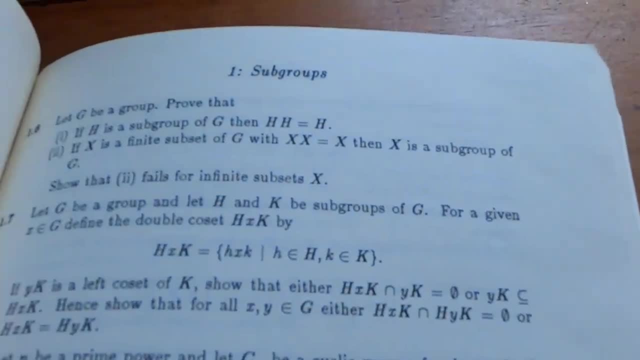 So this has full solutions to problems in group theory. It's pretty hardcore. 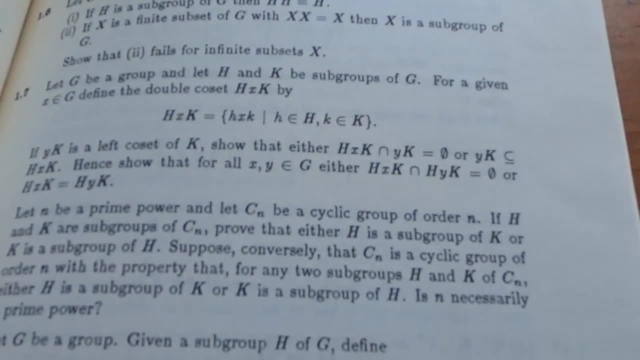 It's got a lot of really good problems. And all the proofs are detailed. 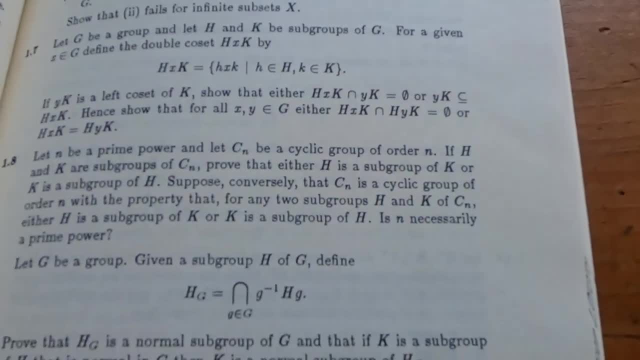 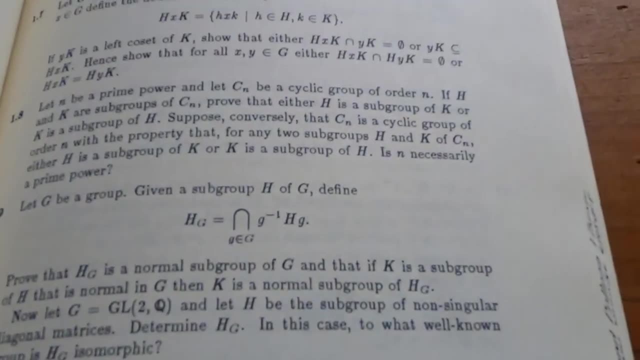 Again, the number one downside to these books from the Algebra Through Practice series is that they are expensive. You cannot get them for only a few dollars. But otherwise, if you can get them, it's totally worth the money. Okay. So this is a really fun book. It's called The Theory of Rings. And it's by McCoy. 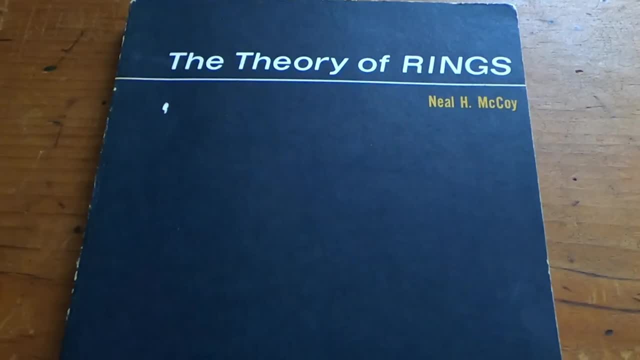 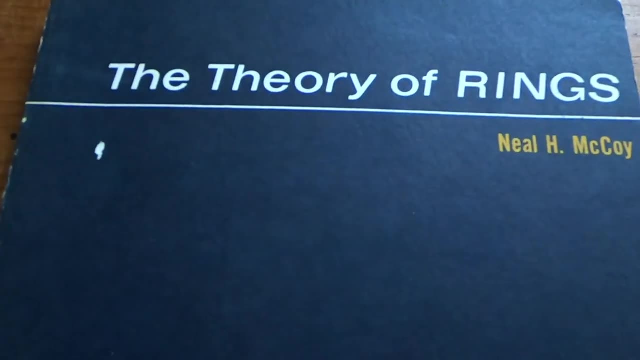 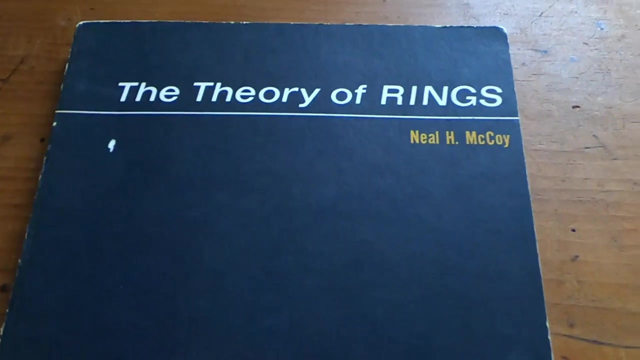 And I say that because you can actually buy this book and start reading it. I mean, it starts from the beginning. It's all about rings. I love ring theory. And I'll probably be making some more ring theory videos in the near future. But this is a book just on rings. It's kind of fun, you know, to have a book just on rings. 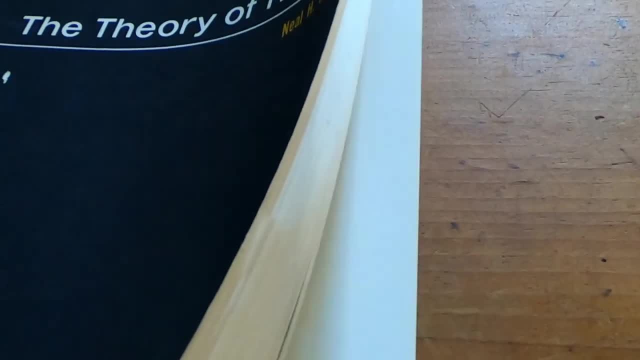 The big downside of this book is that it is a paperback. So, yeah. Theory of Rings. Neil H. McCoy. Pretty cool stuff. So this is a book I actually used for a course. 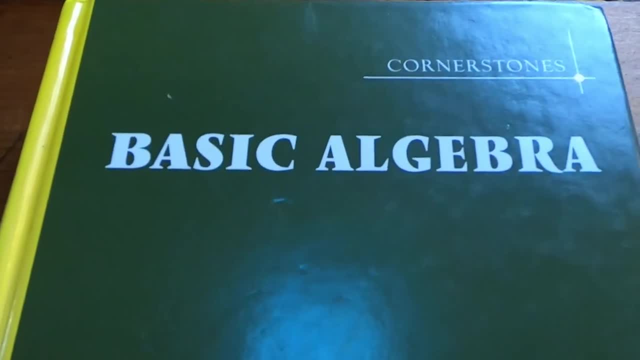 You know, I did some of the exercises from this book because, you know, they were homework problems. This is a graduate level book. Do not let the name confuse you. 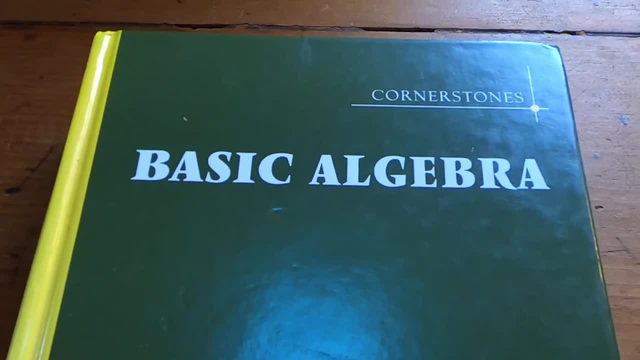 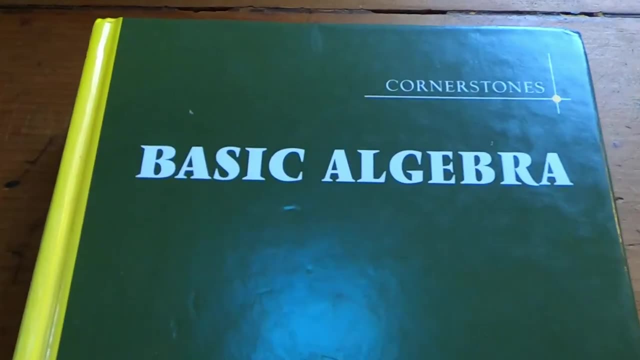 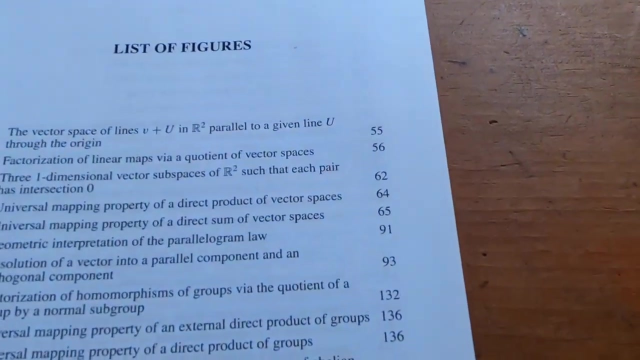 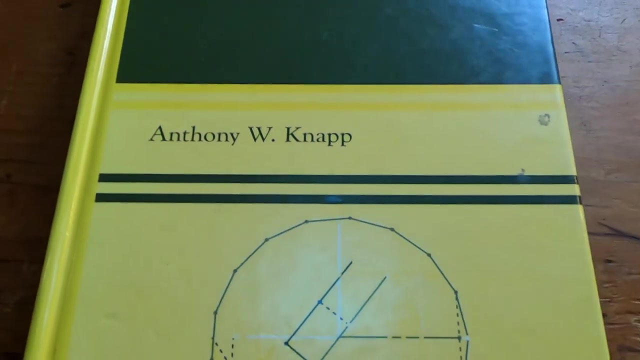 Basic Algebra. I remember I took this to work one day and there was someone in my office. I'm like, oh, Basic Algebra. Is that like, you know, like they thought it was like, you know, quadratic equations and stuff. No, no, no, no. This is a hardcore book. It's got a lot of good information in it. And at some point I will do a review on this book. So decent book, Basic Algebra by Anthony Knapp. 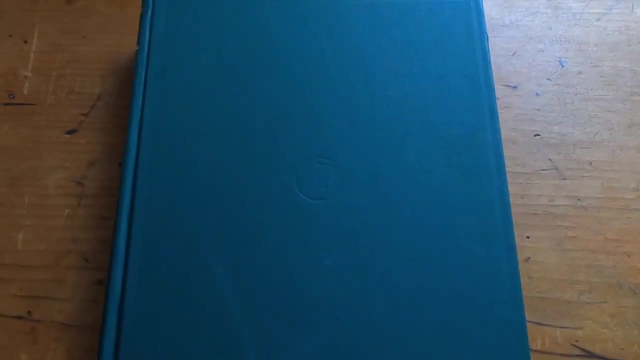 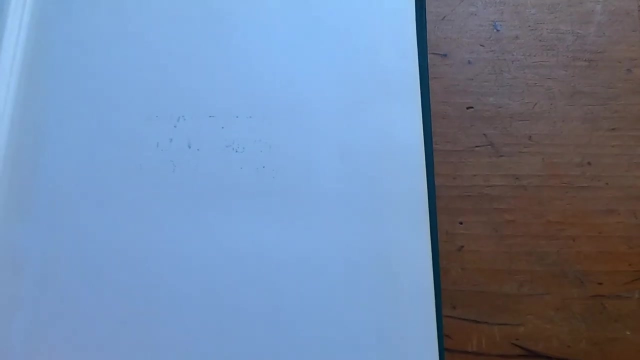 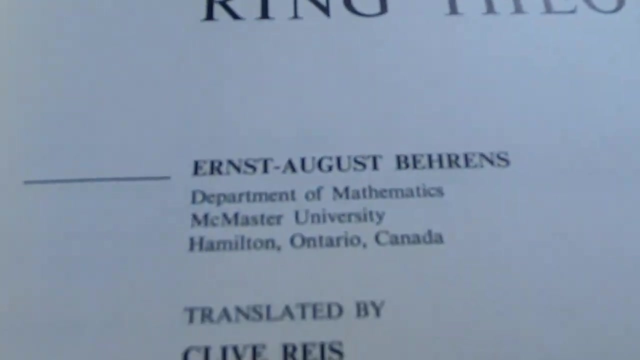 So this is a ring theory book like the one we saw earlier. However, this one does not start as gentle as the other one. This one is pretty hardcore. This is certainly not a beginner book. So the book is called Ring Theory. And it's by Burns. So it's a pretty hardcore book. Let's just briefly, briefly look at the table of contents. So it starts with basic concepts. 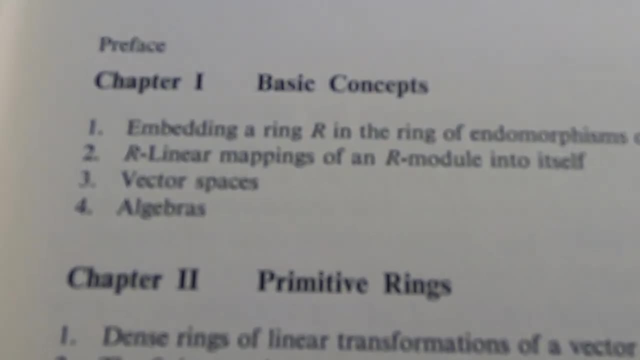 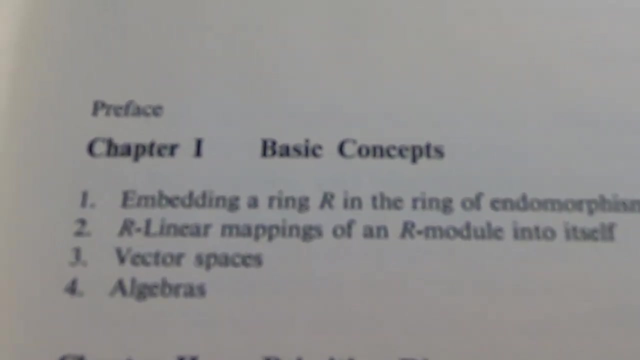 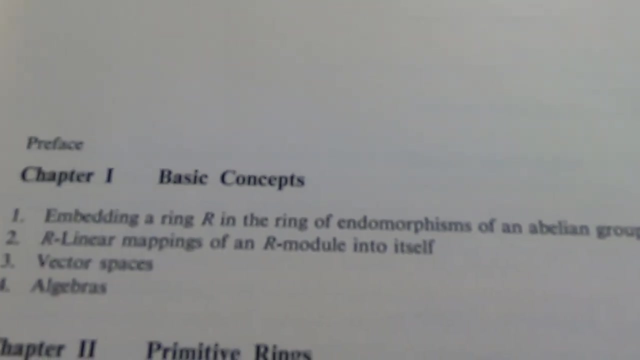 Then right away it goes on to primitive rings. I mean, you see right away chapter one, vector spaces, algebra, algebras, R linear mappings. I mean, already in chapter one. I mean, look, the first section, embedding a ring R in the ring of endomorphisms of an abelian group. That's like the first thing. And the language may not be something you're used to. So it's certainly not a beginner book. 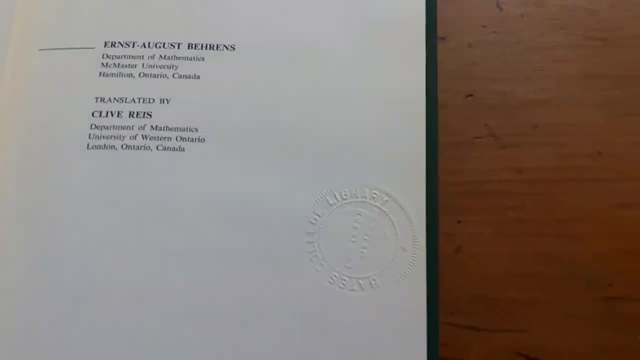 So got Ring Theory by Burns. This book is called Topics in Ring Theory. 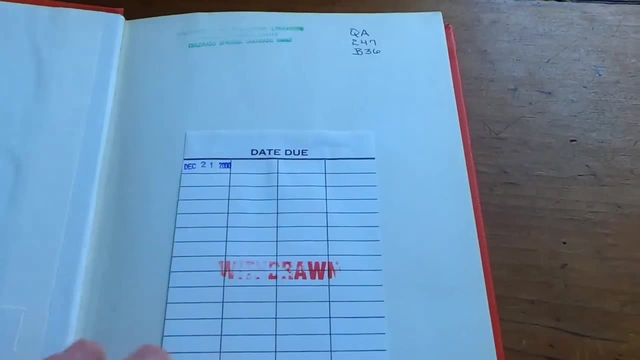 And it's written by Barchet. This is a graduate level book. This is not a beginner book. So this is a graduate level book on ring theory. 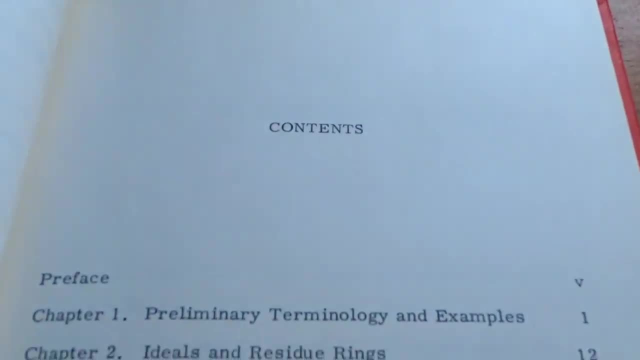 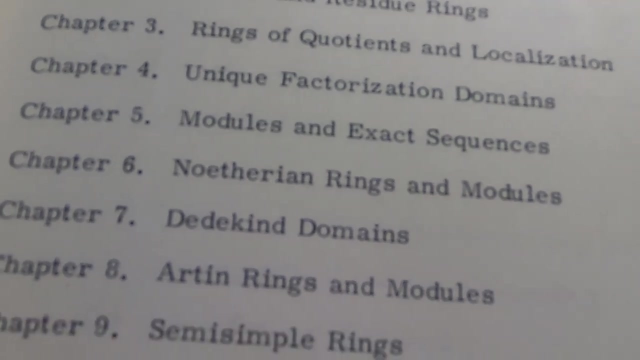 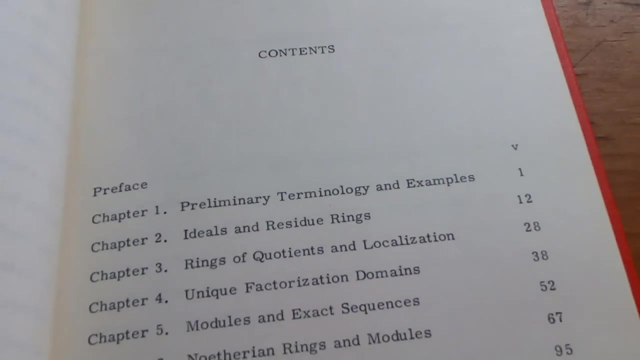 So if you're looking to learn more ring theory and you have some abstract algebra knowledge, it's a good choice. This is the table of contents. So you can see some of the topics are a little more advanced. Than what you would see in a regular abstract algebra course. It's a good book, though, and I've read portions of it. 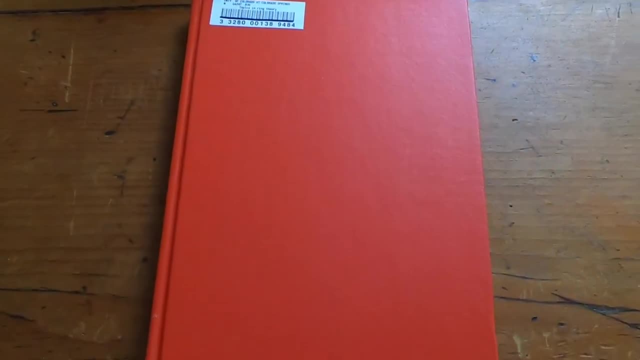 Again, decent choice if you're looking to learn more about rings. 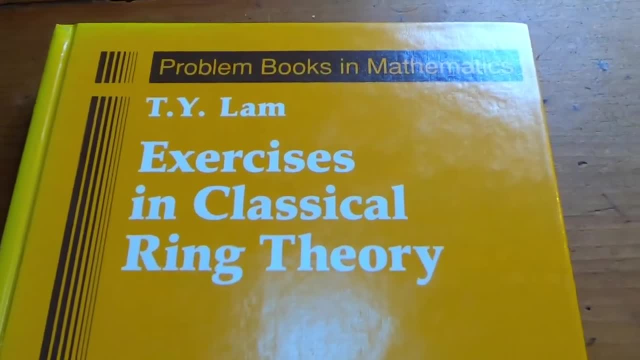 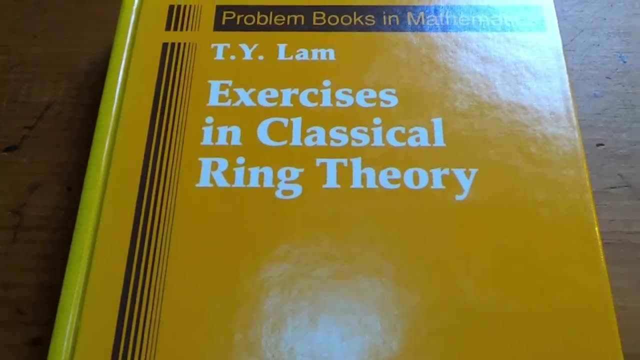 This is an excellent book if you're trying to learn ring theory. Problem Books in Mathematics by T.Y. Lamb. Exercises in Classical Ring Theory. This is actually edited by Paul Halmos. Basically, this book has tons of exercises and they are worked for you. So it's a really, really good way to get into ring theory. 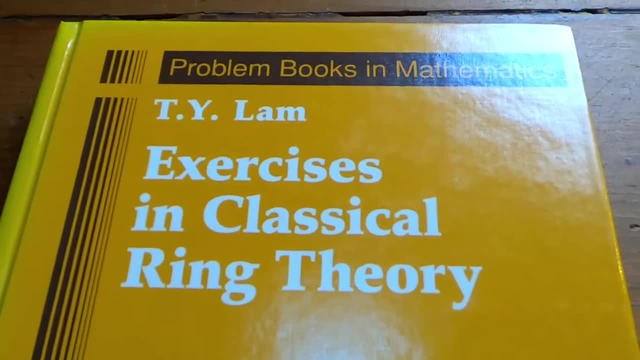 Because you can try the proofs on your own and then when you get stuck, you can look at the solutions. Excellent choice for someone looking to jump into some higher level mathematics. 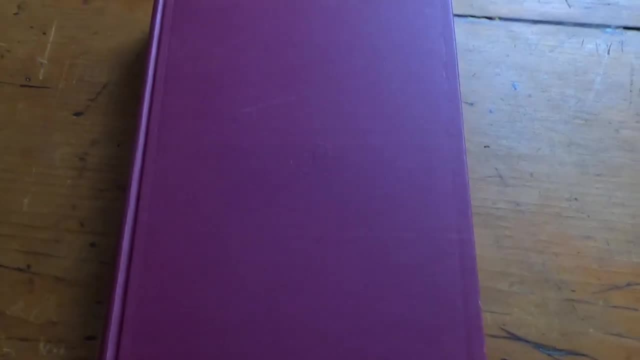 This is another ring theory book. This is Ring Theory by Robert Gordon. However, he didn't write the book. He just was the editor because this is a collection of papers.